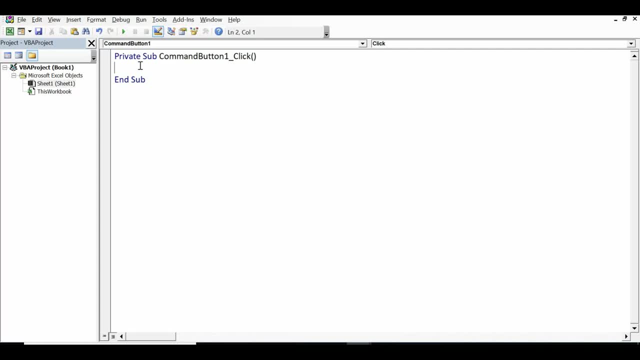 code. first of all, I'll declare two variables: dim my cell as range, dim my range as range, and then I will assign specific range to my range variable. how we can do that? set my range equal to worksheets. then sheet name, which is sheet 1, dot range within brackets and within inverted commas, b3 to h11. once we have. 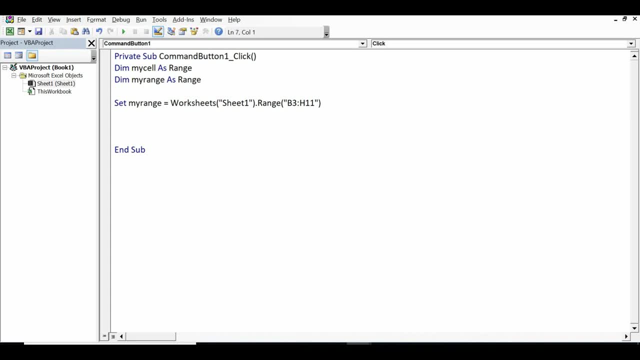 assigned the range. then let me make use of one variable. I'll give name as lowest number. I have not declared this variable, but in VBA we can use any variable without declaring it. so lowest number is name of variable equal to application: dot worksheet function. we have minimum function, dot minimum, within brackets instead of: 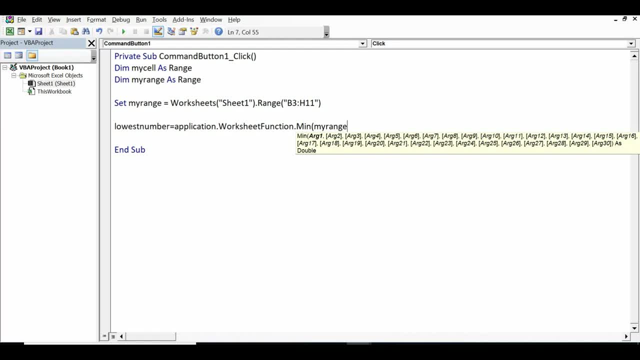 giving any argument, I'll pass here my range. this, my range, has come from this variable. now, highest number. again, this is a variable. without declaring it, I'm using it. application dot. worksheet, function dot. this time I am using maximum function and again I am passing the same range which is there in this variable, my range. and again I am passing the same range which is there in this variable: my range. 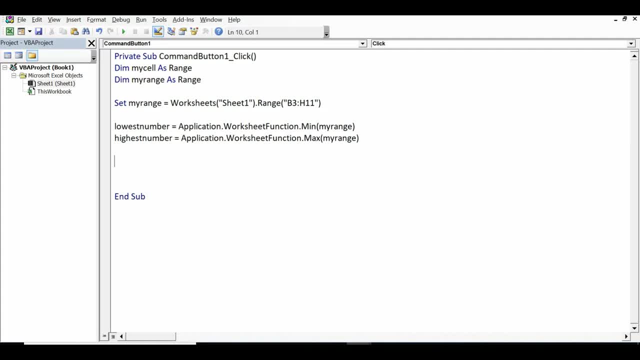 now I will use for loop for each my cell in my range. in closing the statement of for loop, it's particular with in this store looping statement, I'll use if condition or Д, the if condition, $R. if my cell dot value is equal to lowest number, then what we can do is my cell. 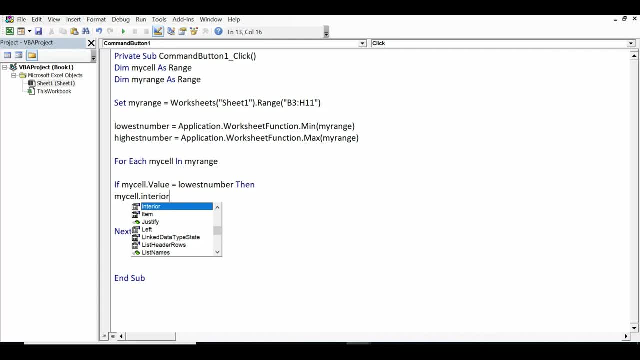 dot. interior dot color index equal to. we can assign any color using a specific number. I want to give green color, so I'll write four here. four is for green color and then closing a statement of: if now I can copy this if condition, paste it here instead of using lowest number. second, 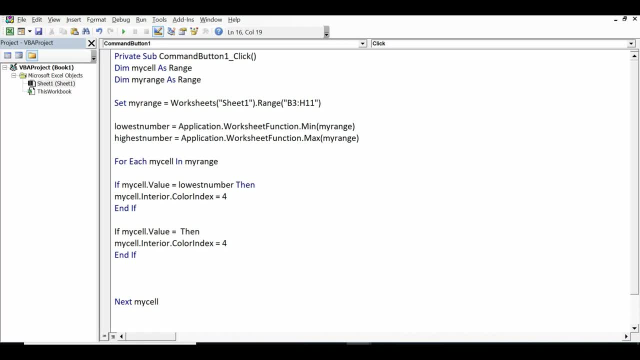 variable I can write. four is for green color and then, closing a statement of, I am going to use which is highest number, and instead of using green color, I want to highlight highest number with blue color, so I'll use five here. now. this is the simple VBA code that we can use to evaluate each cell in a specific range. 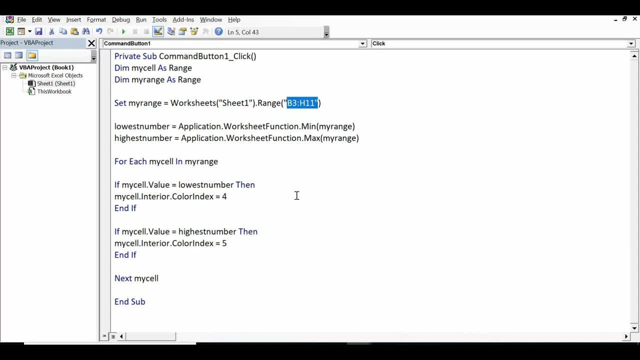 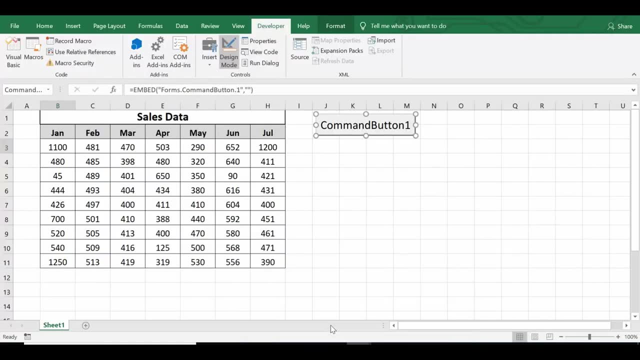 here we have V3 2h11, but we can pass any range that we want. now let me go to Excel sheet. I'll click on design mode and then let me click on this command button. we can see that lowest is 45, highest is 1250. if I make any other cell has lowest, let me 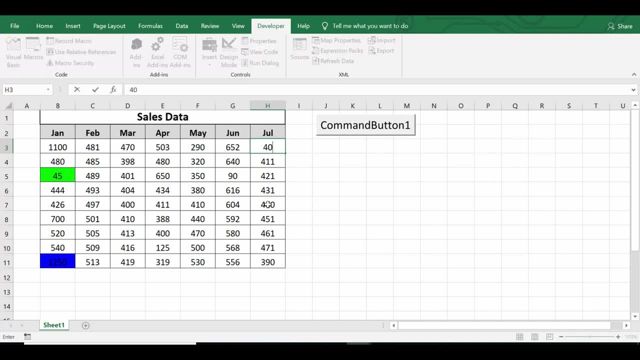 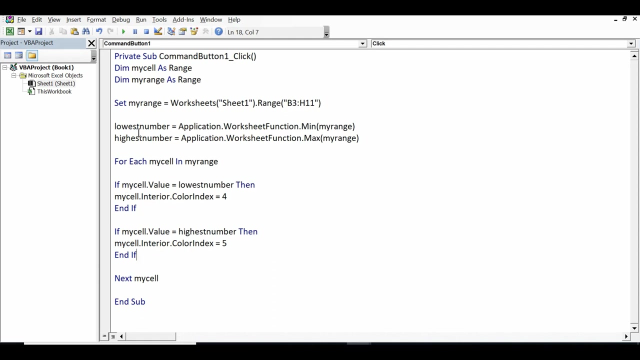 write in h3 as 40 and then I'll click on this command button. so what is happening? new lowest is highlighted, but previous lowest is not removed with color. so to avoid this situation, what we can do is we can add one more line of code. so here: 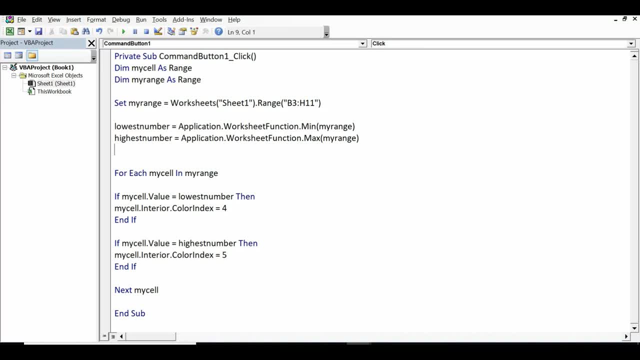 before for each statement I'll write here worksheets, then sheetname: dot range: same range we are going to use. so that is b3 to h11. even we can use the my range variable interior dot color index equal to 0. if we are passing 0 here, that means no. 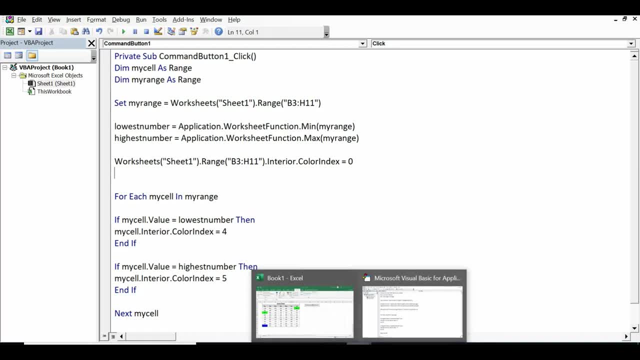 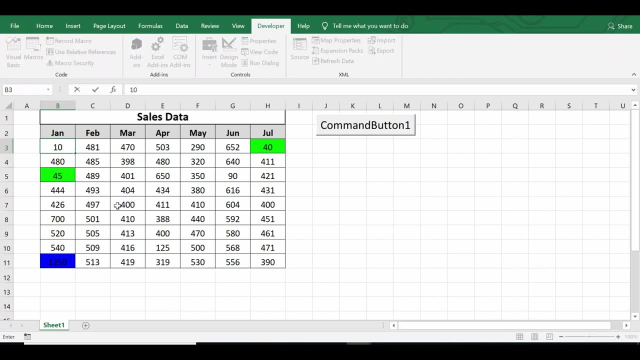 field. now we can check on excel sheet again. if I write b3 as just 10 and then use this command button, we can see that only the lowest number is highlighted. previous lowest are removed with color. and in case if we have more than one cell having same number and lowest, then what will happen? 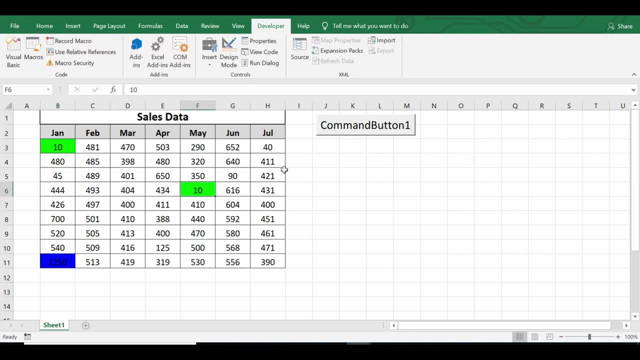 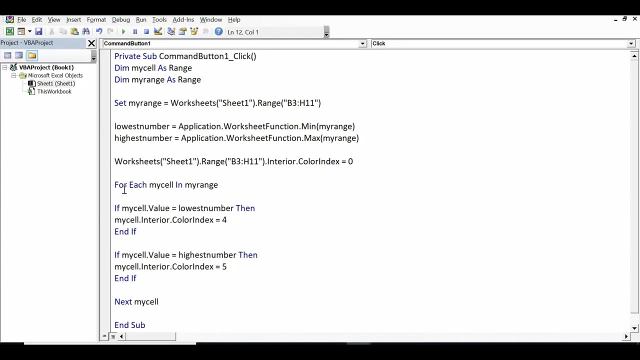 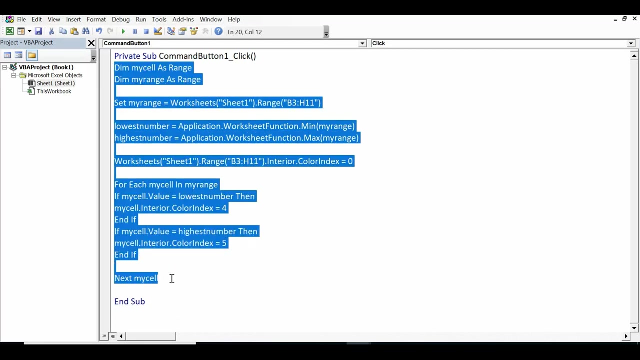 both cells will be highlighted. so right now we are using this code on the click event of this command button. but if we want to completely automate it, what we can do is let me copy this complete code that we have developed. I'll copy this code and then we can see here, instead of command button I'll select worksheet where we